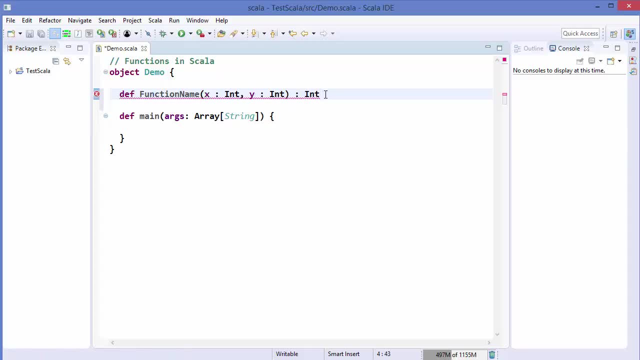 you write the data type, whatever the function is returning right, and then equals, and then these curly brackets in which you write some statement. So let's say we want to add two numbers using a function. So I just give a name: add to this function which takes two numbers. So x and y are two numbers and they are of data type integer. right Now the result. 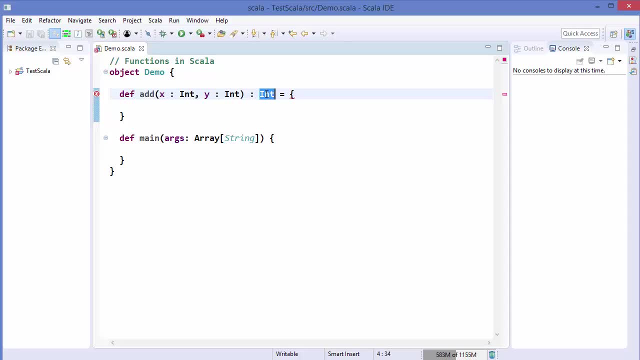 will be return in the form of integer. That's why the data type of result is also integer. and what we can dowe can just write return and then x plus y here. So this is a very simple function which adds two number and returns the result and how you can call that function. For example, I want to print the result of that add function. I can just write: 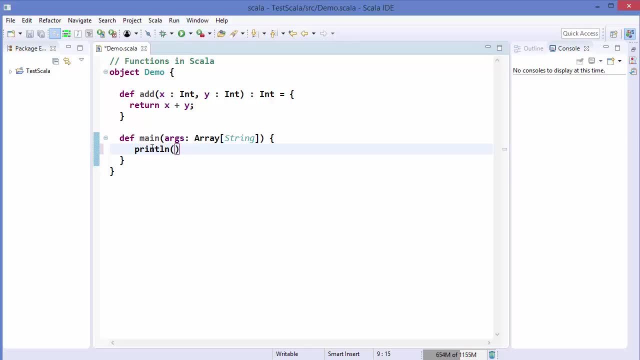 print Ln and then inside that println I can just call this function, for example, add, and then I will just write 45,15, let's say okay, And let me run the code and it's going to give us the result. 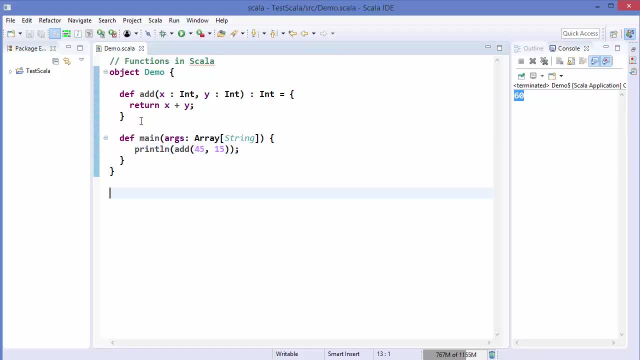 which is 60, the addition of these two numbers. Now, Scala is very flexible language and it allows us to declare a function in different ways. So this is one of the way in which you can declare a function. Let me show you the other way. 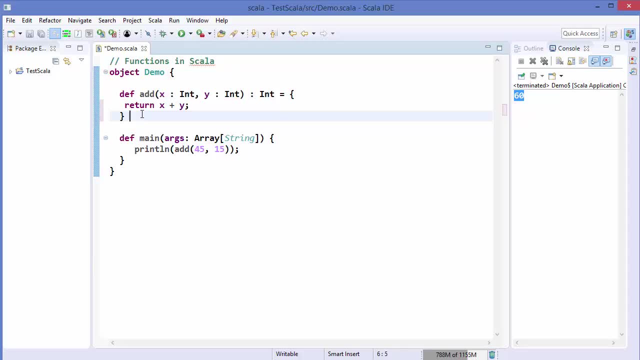 So let me copy this function and let's just copy and paste two or three times, because I want to show you this thing in two or three ways. So let's say I'm going to use a function called subtract and I'm going to use a function multiply. 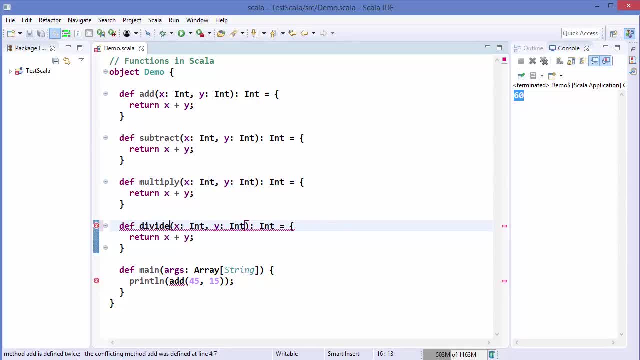 and let's say I want to use a function divide. okay, Every function takes two argument of type integer. Now, as I said, Scala is really flexible, so you can avoid writing this return keyword. Why you can avoid writing this keyword. 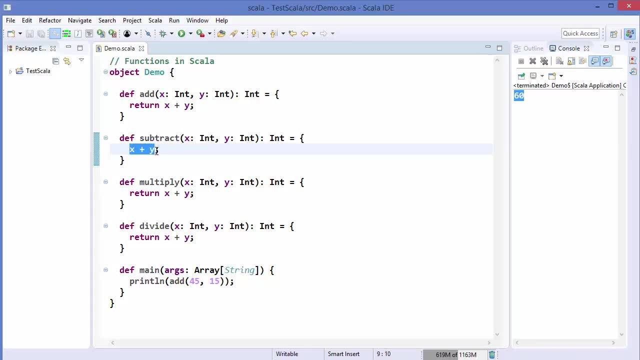 Because whatever is the last line of your function, this will be considered as a return value automatically, if you don't write a return keyword. So here you have a choice of writing this keyword. so you can write a return keyword, Or you can just write it something like this: 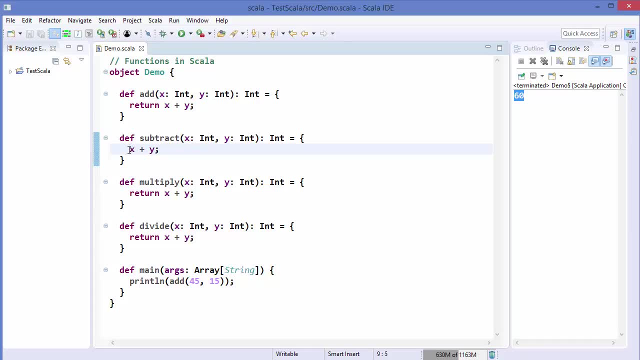 and avoid writing this keyword return and the last line of your function is considered to be our return value. So in this case you only have one line, so it will be considered as a return value, and here we want to do that subtraction. 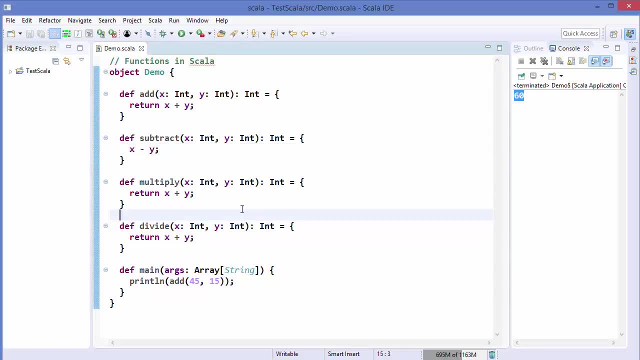 Now, let's say we have a function which is very short and we want to write it in one line, so we can avoid writing it in one line. So we can avoid writing it in one line, so we can avoid adding these curly brackets. 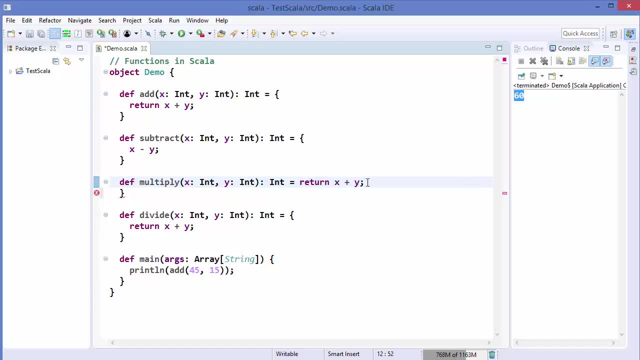 so we can just write this and avoid adding these curly brackets. so something like this: And here you can just write asterisks to multiply, And here you can even remove this return keyword which makes your function more short. right Now, let's make this divide function also the same. 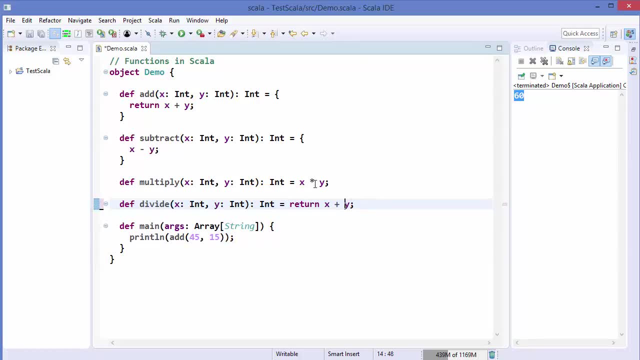 So I'm going to remove these curly brackets from here and then I'm going to also call it one, 그렇죠, I'm going to want to do it again in the next period. So remove the return keyword and then I will add this forward slash to divide x by z. 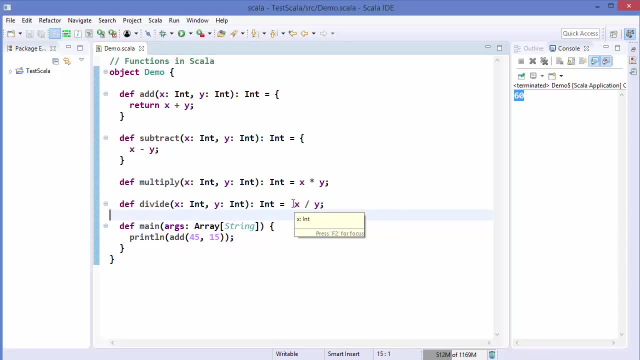 Now, in cases where Scala is certain that it's going to return a certain type of value, certain data type of value, then you can avoid writing the return data type also. So, for example, we are certain that this divide function is only going to return an integer. 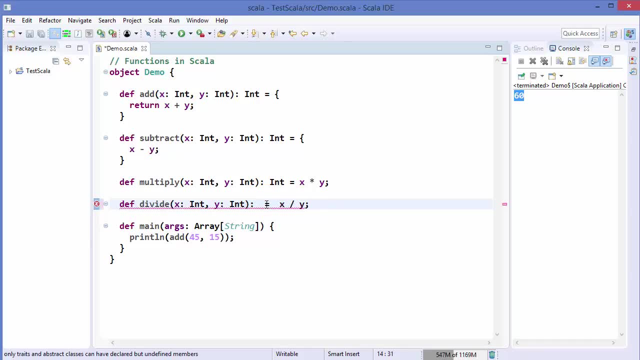 We can avoid writing this return value, and then we can even remove this semicolon. Okay, so that makes our function more shorter and concise. So these are the four basic ways of writing a function in Scala, And now let's call all these functions. 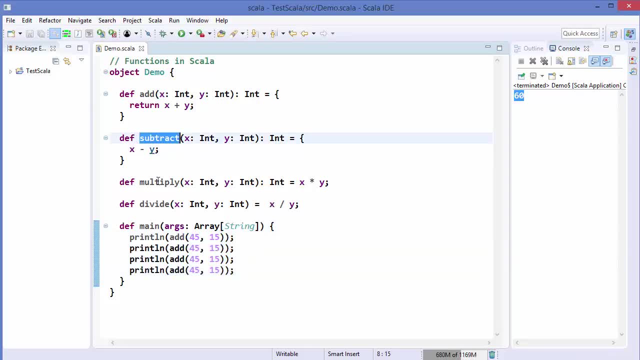 So I'm going to just call the subtract function here and then multiply function here and then divide function And let's see what's the result we get. So you can see, these are the result we get from these functions. Now let's say we create an object. 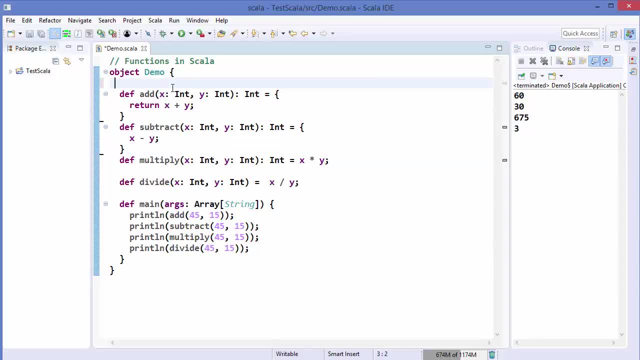 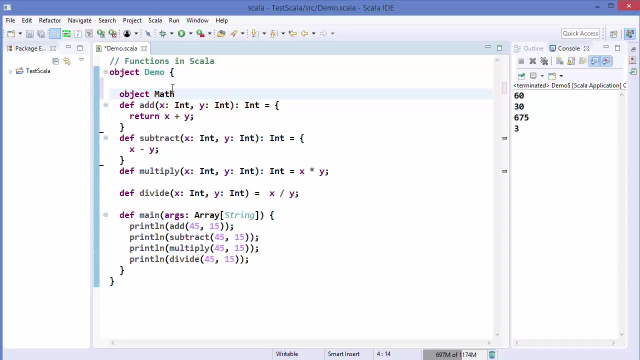 So I'm going to just create an object at the top. Let's say we have our object, We declare our object and the object name is math, in which I want to just include all the math functions, right. And let's say we have a function here. 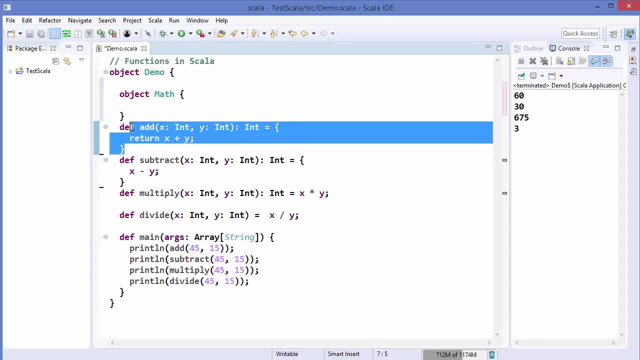 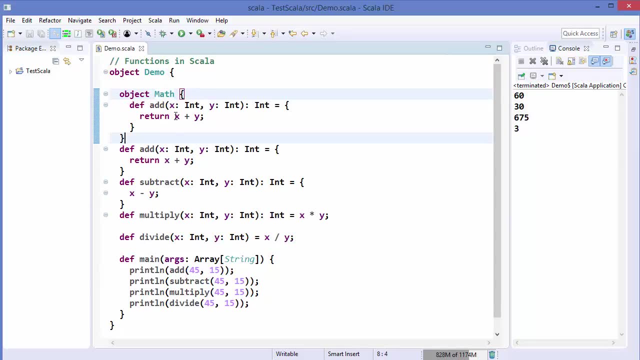 We have this add function inside this math object, So I'm going to just copy this add function and paste it inside the math function. Now how I can use this add function from this math object. So it's really simple once again. so I can just write print line and then I can just 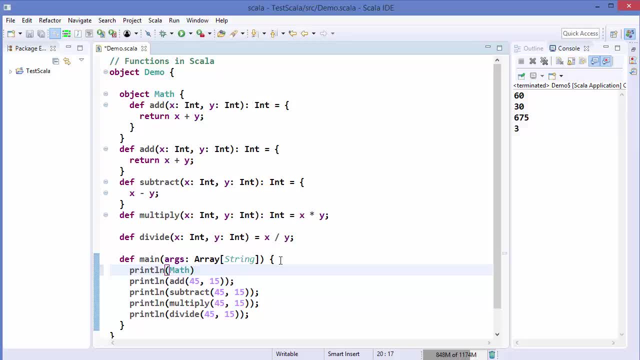 write math, which is the object name, dot the function name, which is add, and then the argument which it takes for. so, for example, 45 comma 15, and then just close the print line parenthesis. Okay, So because it's an object, we don't need to create a new instance of this object, right? 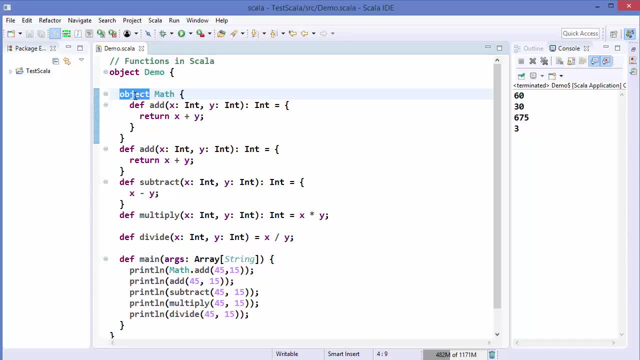 So if it's a class, we need to create an instance of this object with a new keyword. but because it's an object, we can directly use dot operation. Let's create a new function on this object and then call the function which is inside that math object. 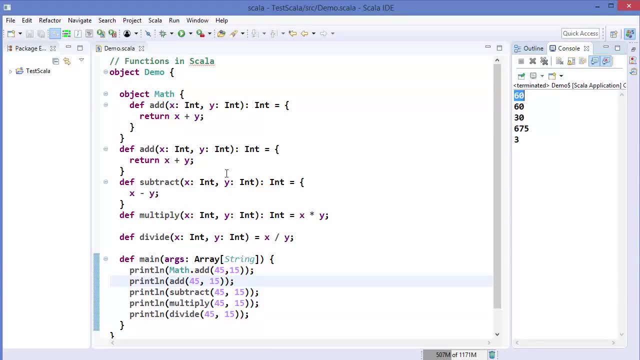 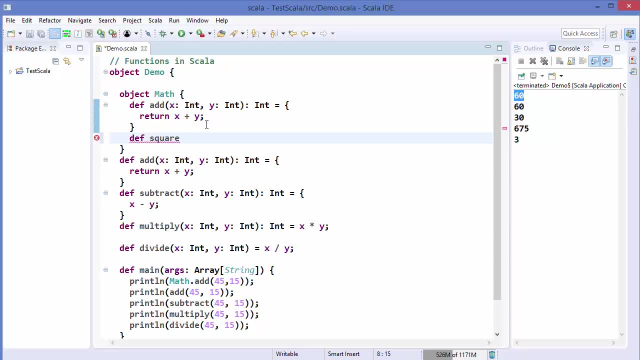 So let me run the code once again. it's going to print the value of that function once again. Now let's say I have a function, let me declare a function, so def square, and this function only takes one argument. So let's say it takes one argument of type. 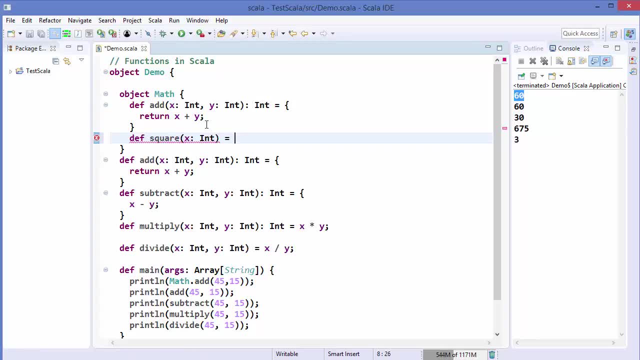 Int returns the value. so it will return equals X multiplied by X, which is X square. okay, so the function which only takes one argument. we can use the syntactical sugar with these functions. so, for example, let me just copy and paste this here and then this square function here. so math dot square and 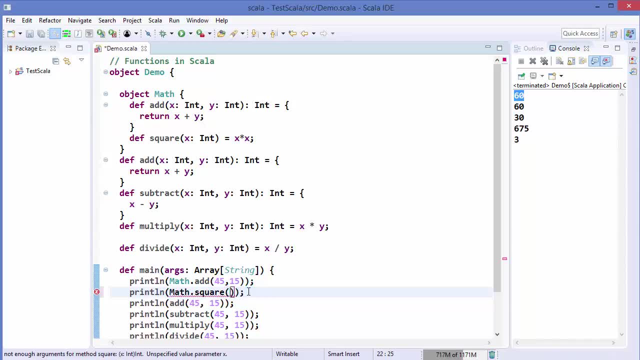 let's say we just give 3 here as an argument. we can use it something like this: so it's going to give us the square of 3. you can see like this, or you can use this notation: so math space and then square space and then whatever you want. 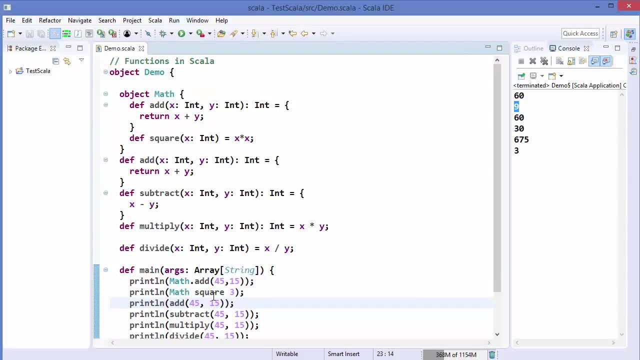 to give as an argument. so this is also a valid operation, right? so if the function has only one argument, you can write it something like this. so you can write it something like this, this: so math space, square space, whatever the argument is, and it will work perfectly fine. you can see, it works perfectly fine. so this is the